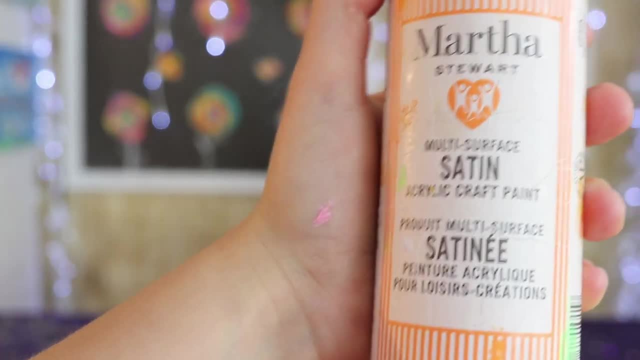 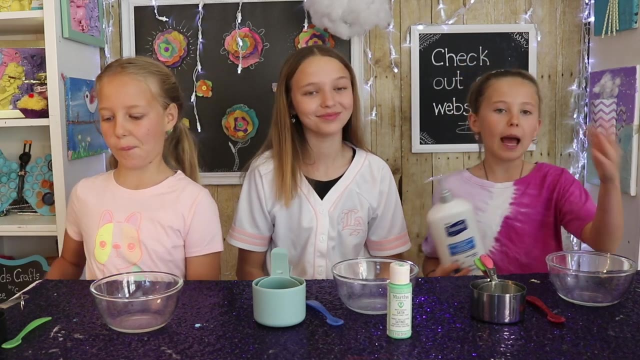 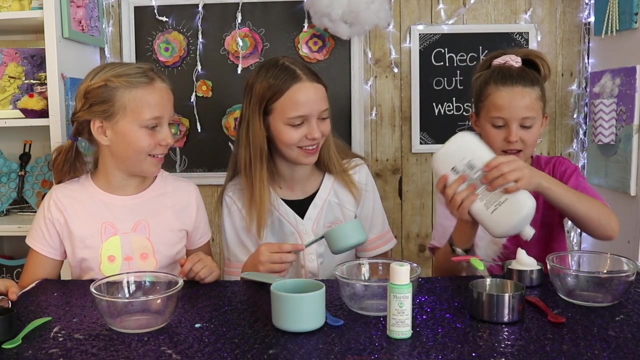 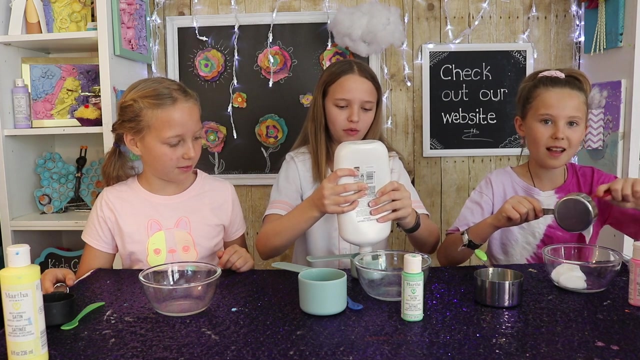 cup of lotion, one cup of cornstarch, paint of your choice and a mixing bowl. So the first step to make cloud dough is to take half a cup of lotion and put it into your bowl. Make sure you get the cheap brand from the store so you're not wasting your. 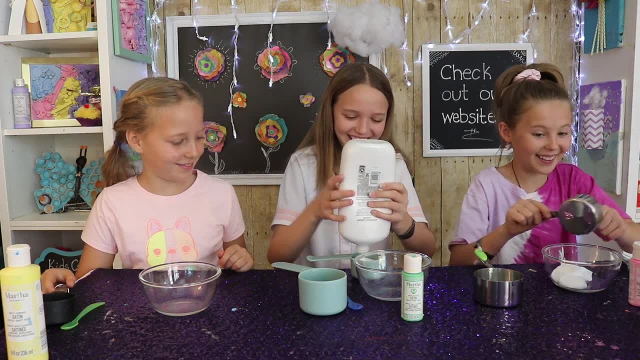 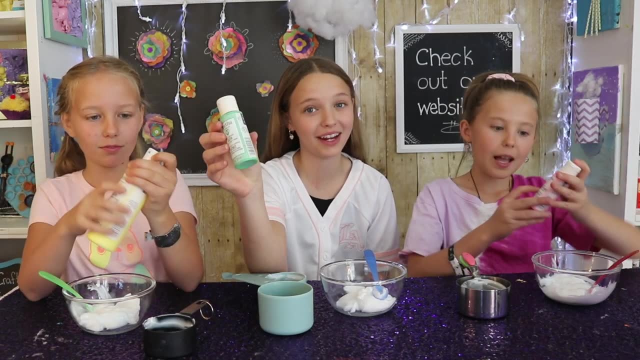 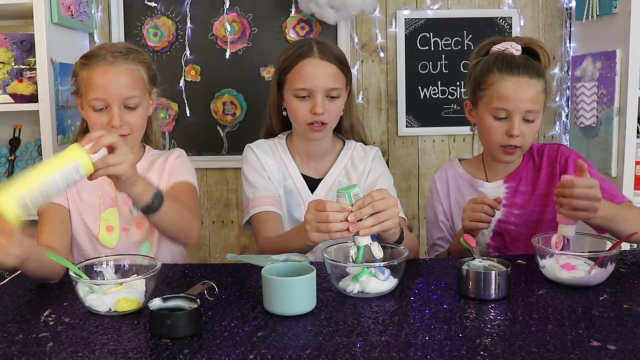 good stuff. The next step is to put your paint into your lotion. I'm doing green, I'm doing pink And I'm doing yellow. You can do however many squirts you want, It really doesn't matter. Yeah, but the cornstarch will make your cloud dough lighter. 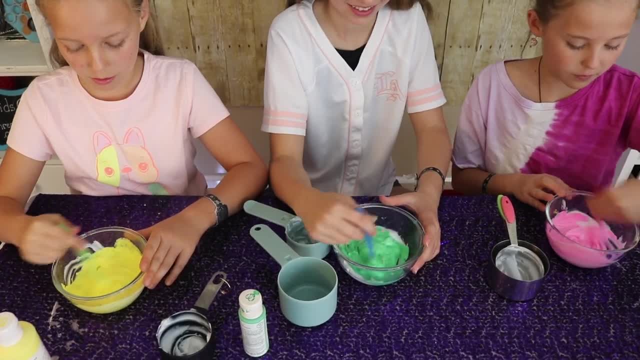 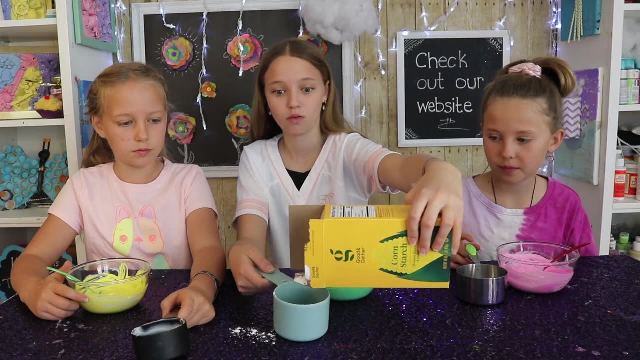 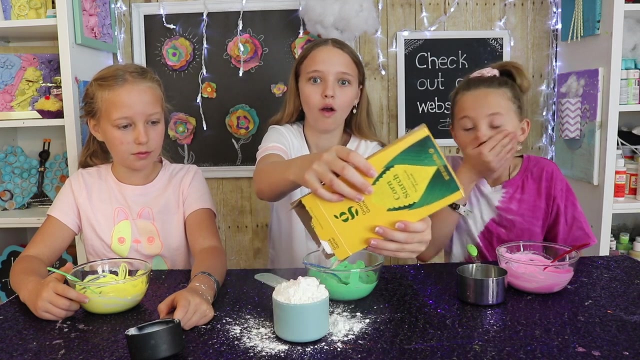 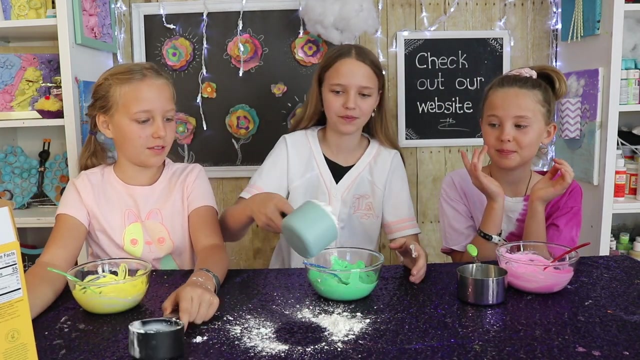 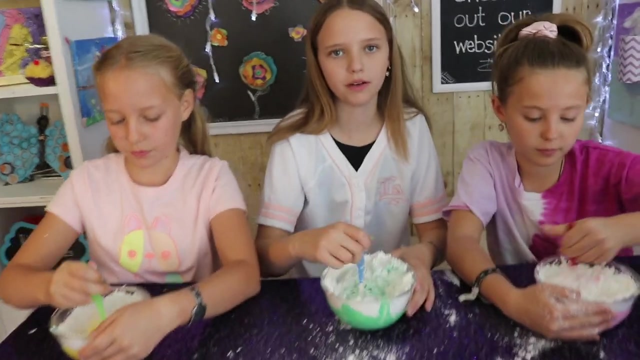 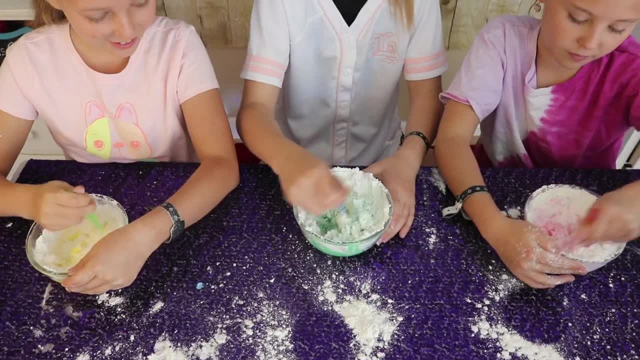 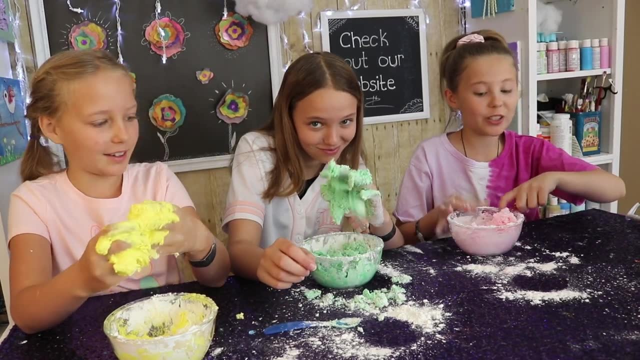 Now we're just going to mix. Don't be afraid to get messy kids. That sounded so animated, Mom, it looks like eggs. Once you're mixture starts to look like this, it's time to put your hands in. Oh, So funny. 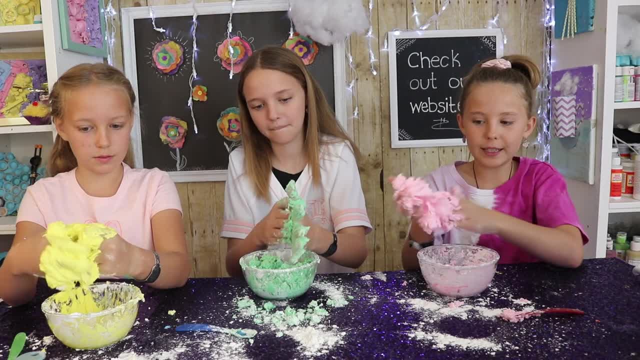 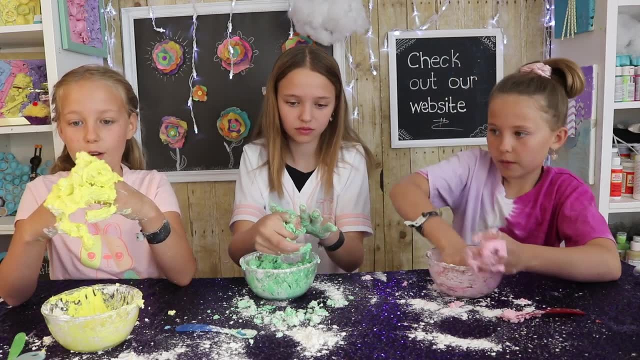 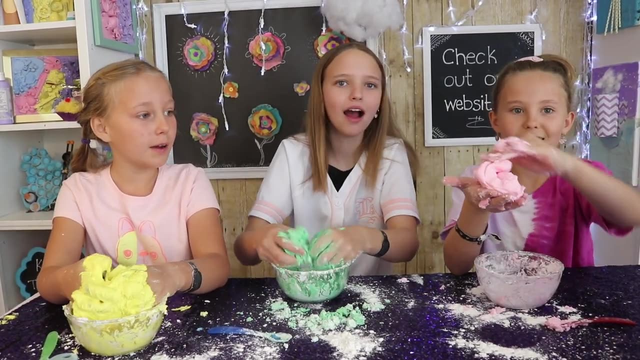 Oh, So fun, your mixture, and it starts to feel a little bit sticky, like it's sticking to your hands. you should add a little bit more cornstarch. mine's not feeling sticky, it's feeling wet. it'll look like this: i want mom, i need corn. what did you guys do? mine is too liquidy, so 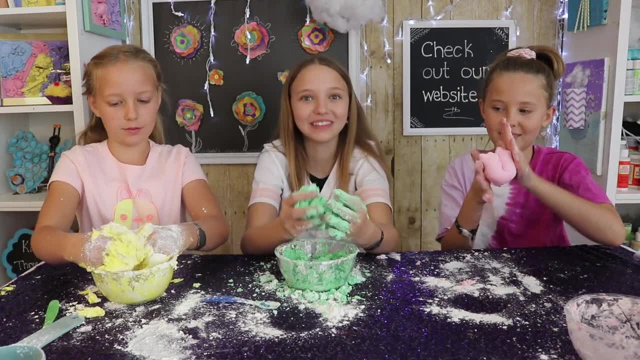 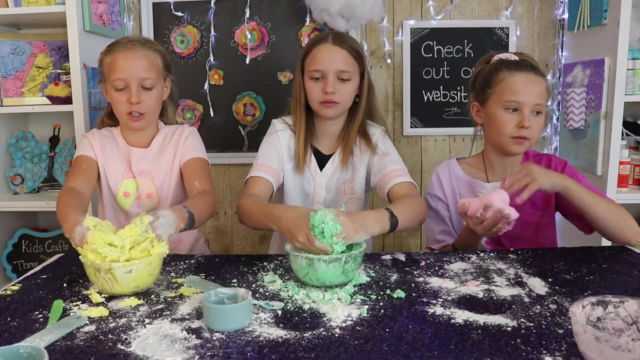 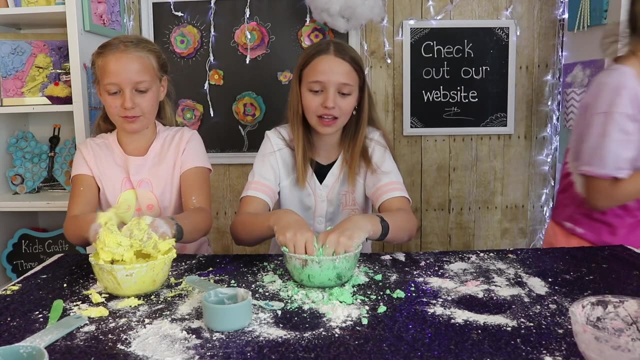 i'm going to add more cornstarch and mine's way too crumbly, so mine is perfect. hey guys, welcome back to the kids crafting championship guys. i look over at brenda's plate and hers isn't going so well. then i look over at kashi's plate and hers is really good, so i'm